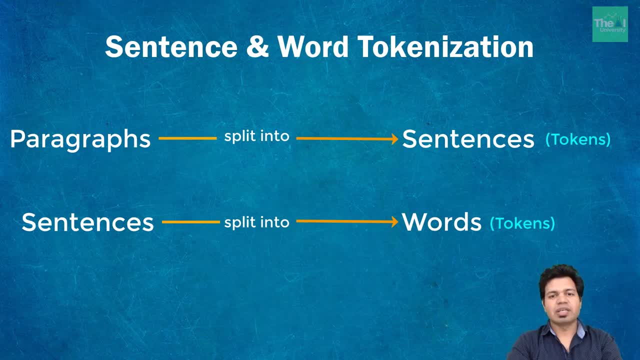 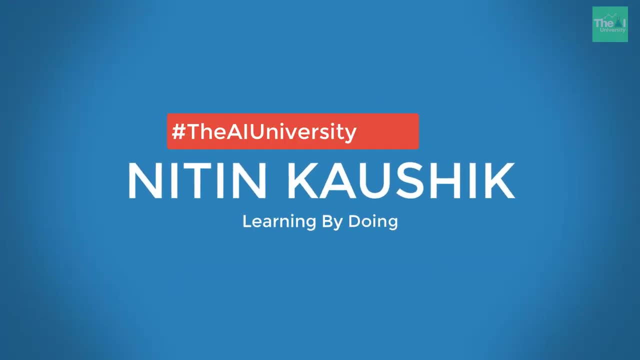 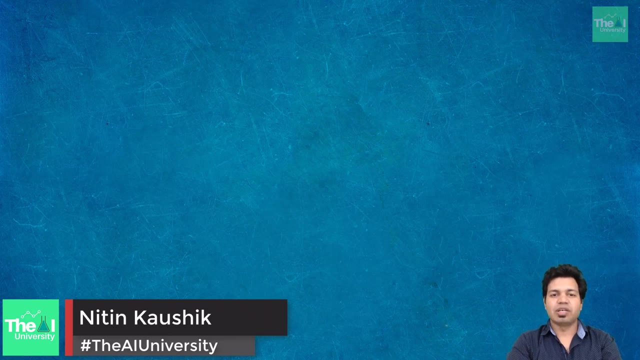 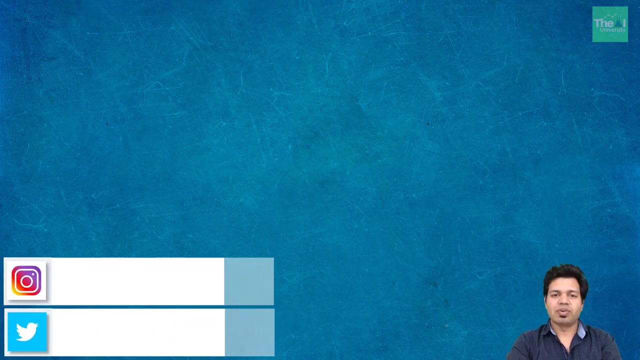 processing, So please watch this video till the end to get the complete details. Folks, this is Nitin welcoming you to AI University channel, where you can learn all your favorite technologies like machine learning, deep learning, AI, big data, Hadoop, virtual reality and cloud computing, and you can acquire the 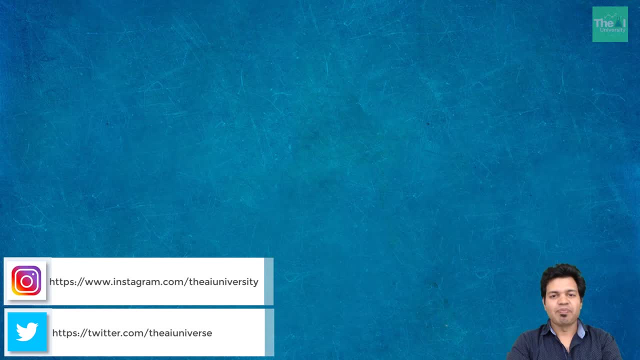 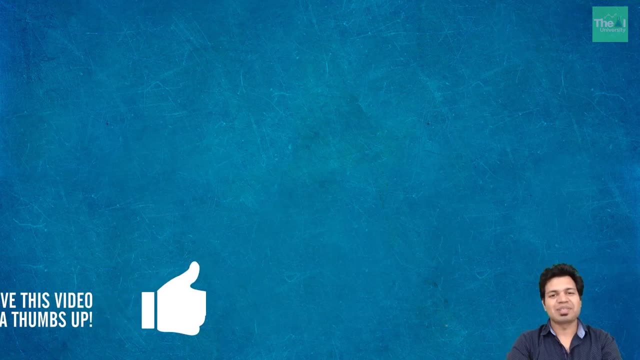 related skill set in order to advance your career in these fields. This channel takes on hands-on approach to build AI based products and applications. so if you are new to this channel, consider subscribing to it, or if you have already subscribed, then click on the bell icon to receive the. 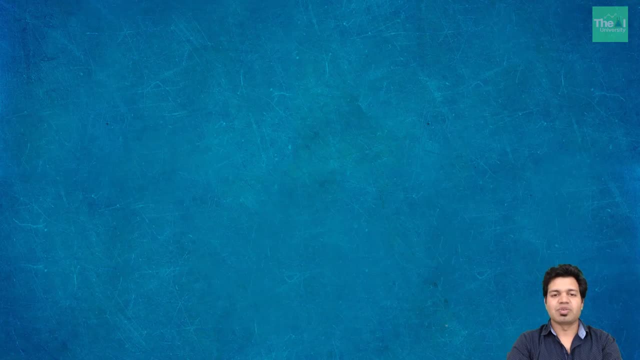 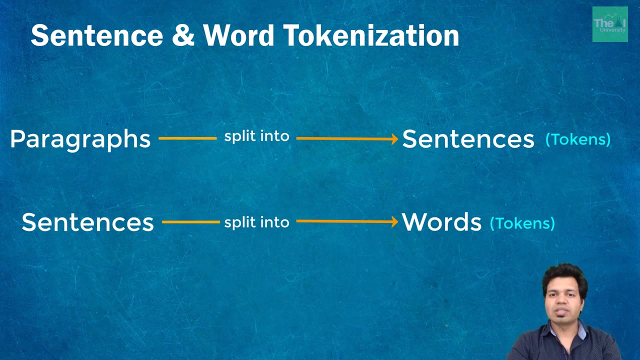 notifications about the hottest technologies of 21st century. So tokenization is the process of segmenting or slicing text into words or sentences. Essentially, it's a text processing step which assumes splitting text into tokens such as words or sentences. Okay, so you can use some kind. 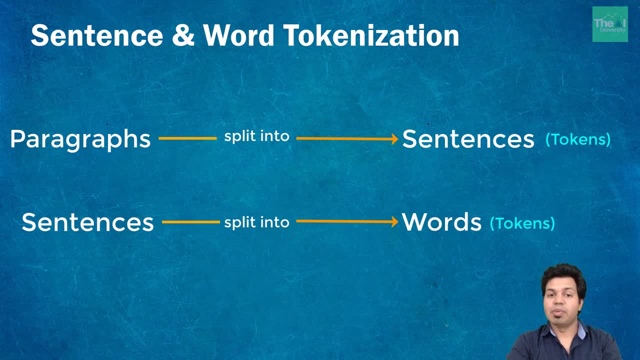 of simple separator to achieve this splitting. but don't forget that there are a lot of different situations where separators just don't work Okay, and when I'm saying separators, I'm talking about you know, those spaces between individual words or comma okay, or dot such and you 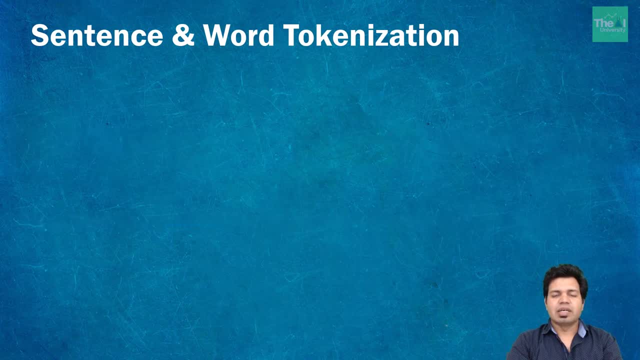 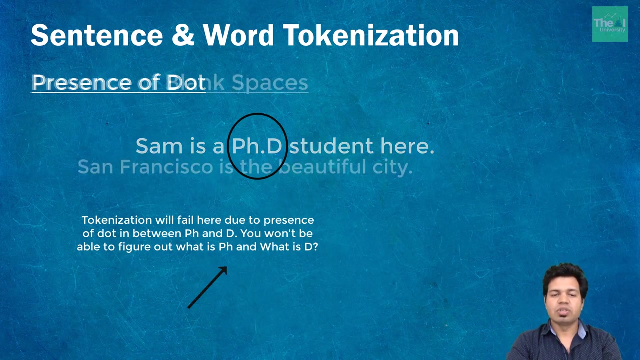 know so and so forth. So, for example, let us say we have a dot separator for tokenization into sentence and it will fail if you have- you know, every video variations with dots. Okay, another example is of blank spaces in English language. So blank spaces alone are not sufficient enough for English to perform. 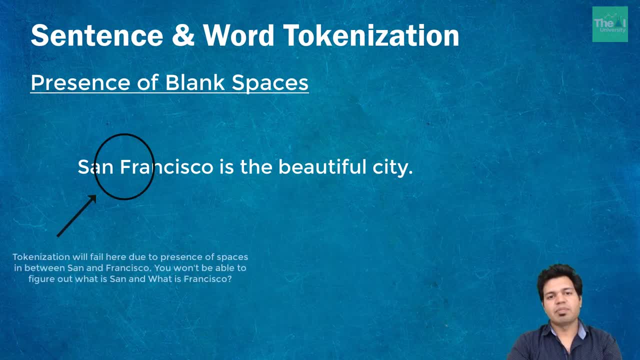 proper tokenization. Splitting on blank spaces may break up what should be considered as one token, as in the case of certain names, For example. let's say we have a city named San Francisco or New York, So if you use spaces here, it will. 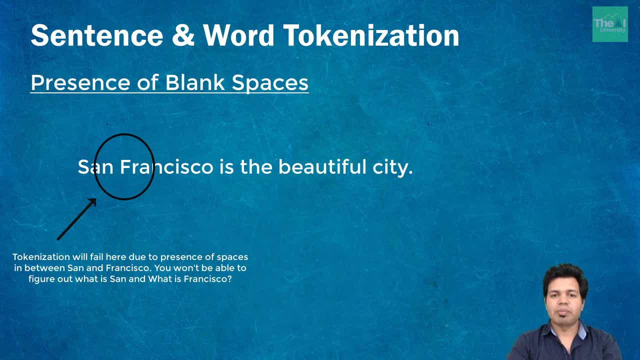 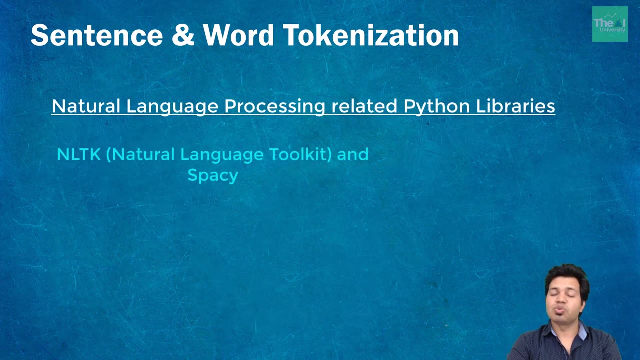 separate out these individual words into separate tokens and you won't be able to guess the meaning out of it. Okay, so you have to have more complex model to achieve good enough results. Okay, and we use NLTK or a spacey NLP libraries to. 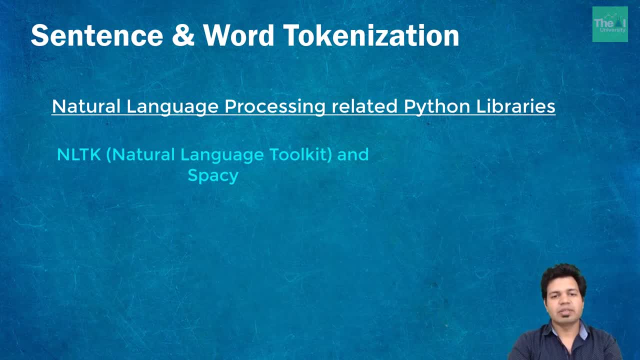 achieve some of the complex tasks right. So, without further delay, let me show you the Python code involved to perform that tokenization. Okay, first I will show you how to perform sentence tokenization and then later on, I will show you how to perform the word tokenization. So let's start sentence. 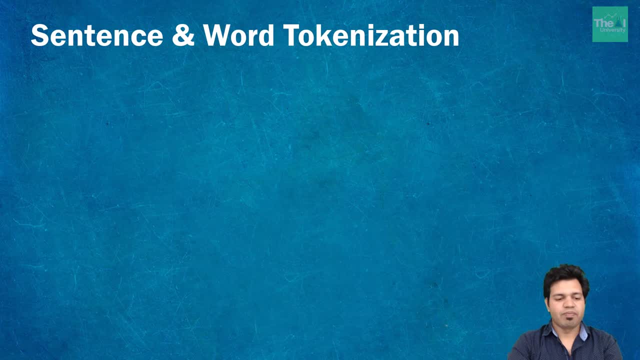 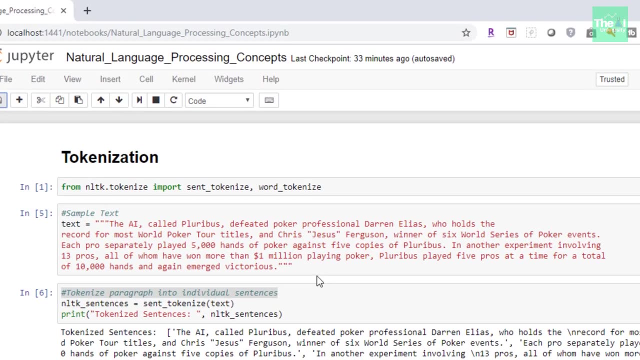 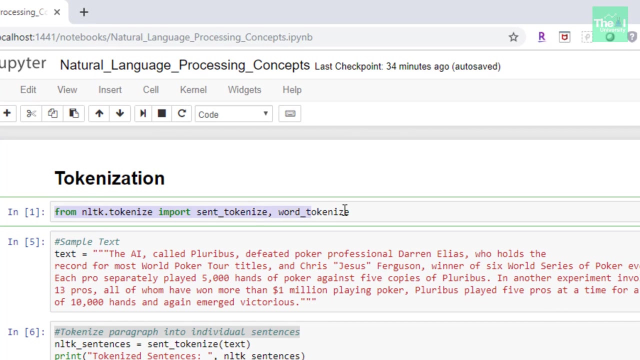 let's start with sentence tokenization. Okay, so let me open my Jupyter notebook here real quick. So first of all, I imported, you know, all I imported this sentence tokenization and word tokenization from NLTKtokenize. Okay, so this is the first statement and you know I have then used this sample text for. 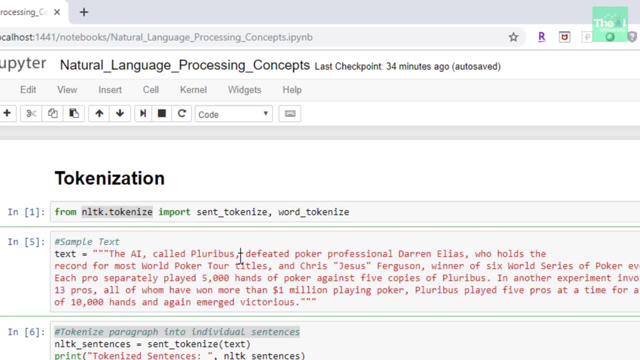 breaking it into sentences as well as individual words, using these methods, like sent tokenization, which will be used for sentence tokenization and word tokenized for word tokenization. Okay, so this is my sample text here and now, in order to, you know, tokenize the sentence, I used this method called. 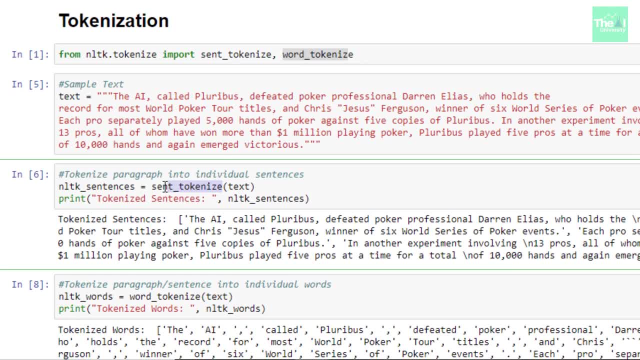 sentence sent tokenize. Okay, this is the method: sent tokenize, as shown here. Okay, and what I'm doing here is I'm just using this method and passing this text, which is the sample text, as an argument. Okay, and when I print this, print this tokenized NLTK sentence, we can see that our entire paragraph has been. 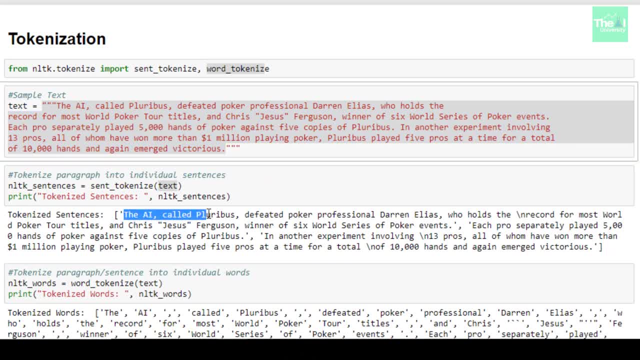 split into individual sentences. So you can see that this is a single sentence which is separated by comma. So comma is a separator for each. an individual sentence here. Okay, so this is the first sentence. This entire paragraph has been broken down into individual sentences. This is the first. 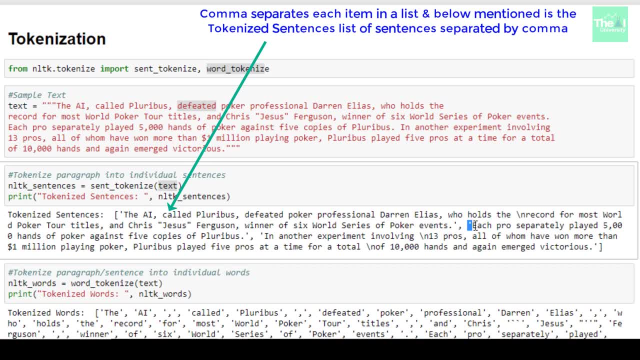 sentence. Okay, and then next sentence starts from here, because we have a comma separator here. Okay, and this is ended here. So this is our second sentence and this one is our third sentence. Okay, so you can very well see that sent tokenize method has split this particular paragraph or text into. 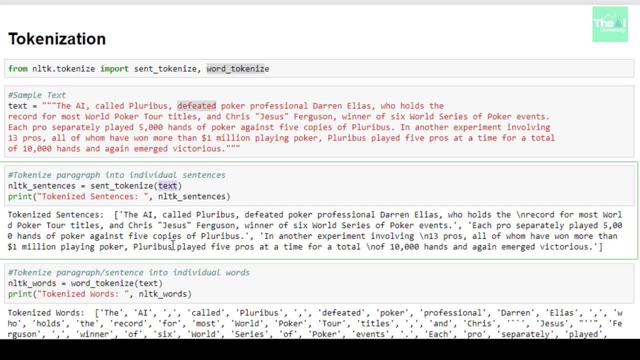 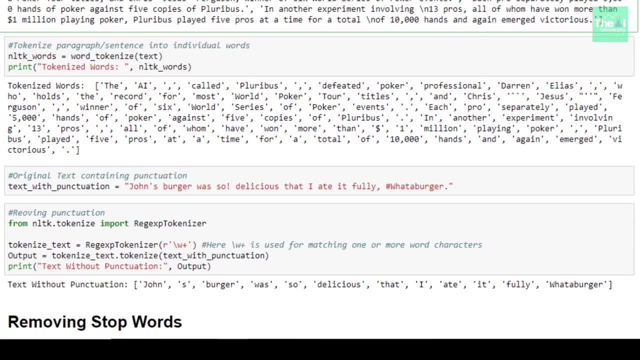 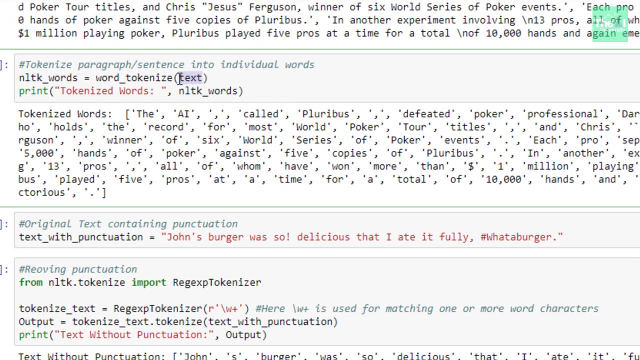 individual sentences. Okay, now let's move on to the word tokenization. Let me scroll down So here you can see that. you know, you will observe that this is the same text which I'm going to use here as well. Okay, and the method which I am using here is word tokenize, which is: 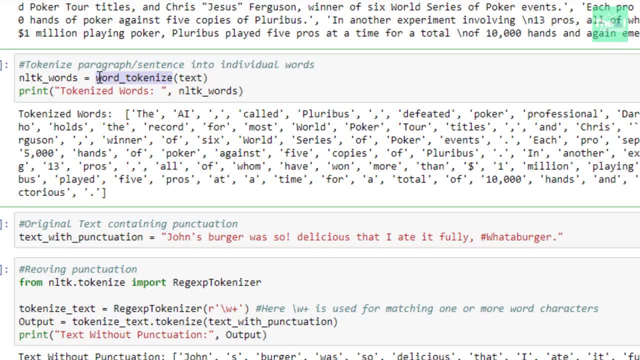 a method to tokenize the sentence into words or paragraph into words. Okay, and again I passed the text as an argument to this particular method. Okay, and in the output you can very well see that the tokenized words are here. Okay, so each of these single words are treated as tokens, Similarly, above each. 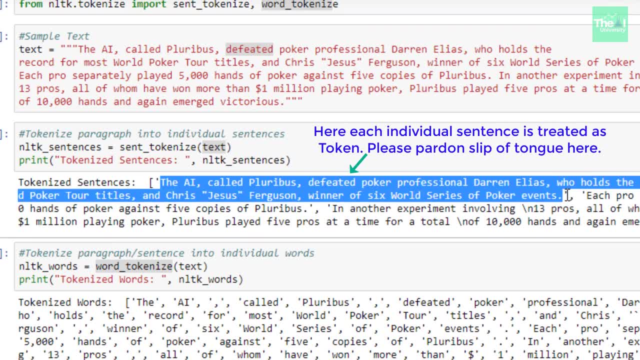 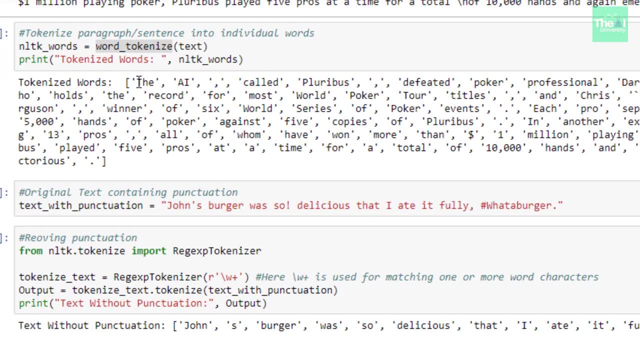 of these individual words are called as tokens with respect to sentence tokenization, and if we are talking about word tokenization, then the each individual words are referred as tokens with respect to word tokenization. Okay, So you can see here very well. Now, if you see here, you will observe there are a few. 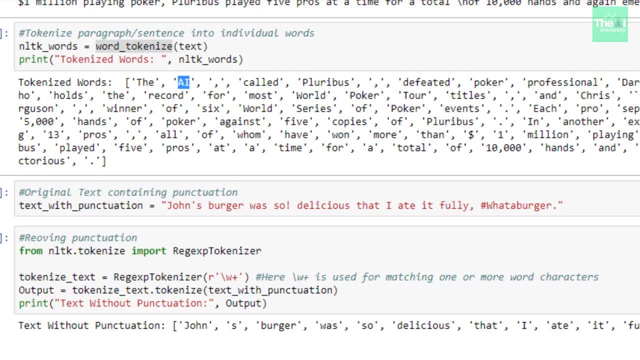 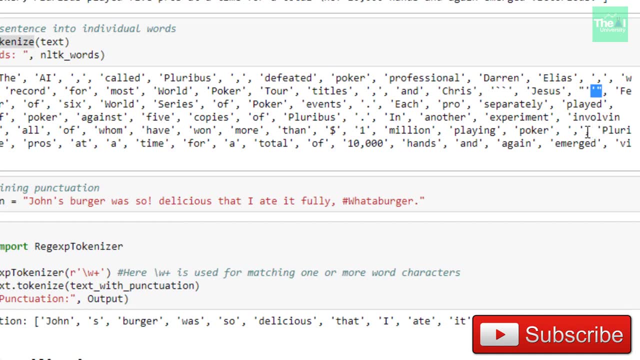 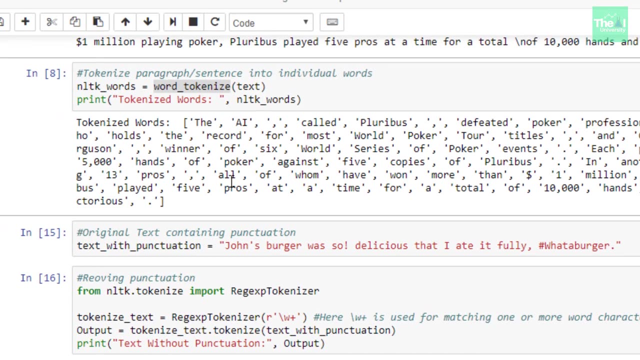 punctuation characters as well. Right, So we have this invert, you know inverted commas here. then we have comma here, punctuation Okay, so on and so forth. So we have several punctuation in this particular punctuation marks in this particular Okay. Okay, So this is what we call the word tokenization list. Okay, If we have dots as well here. 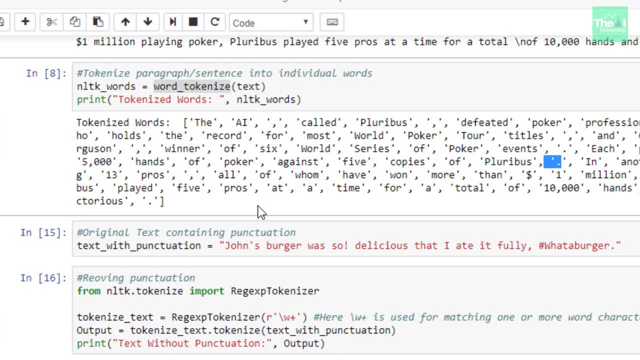 Okay. So we consider cleaning up- you know as well here, which will remove all the undesirable contents. We generally remove punctuation when punctuation does not bring additional value for text vectorization. So it's better to remove punctuation after the tokenization step because doing it before the tokenization is complete. 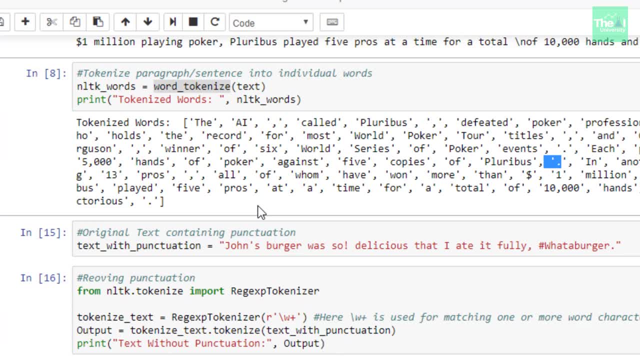 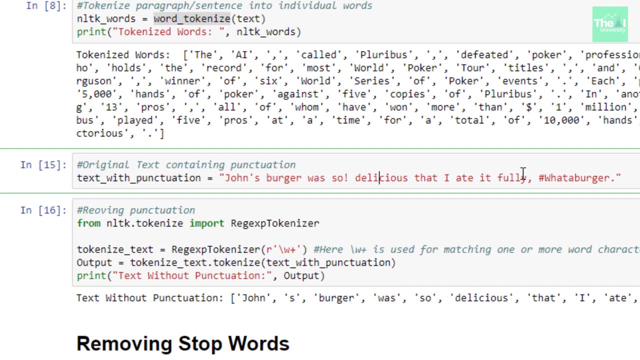 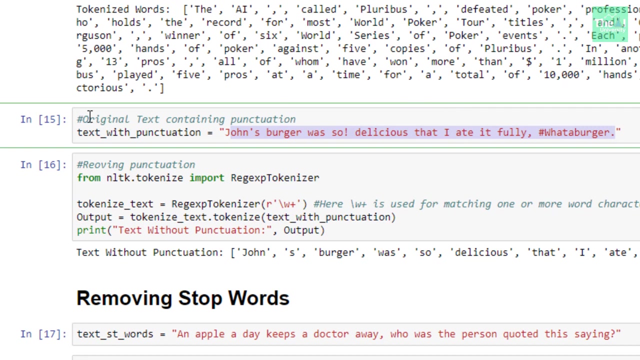 Okay, might cause several issues. so, in order to remove punctuation, I have used a- you know- different sentence here. okay, so this is my sample text and now I want to remove the punctuation from this particular sentence or text. okay, and the way I do it? and, as I mentioned earlier, it's always better to perform this. 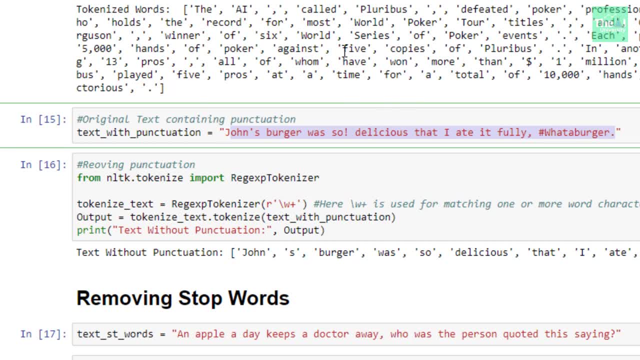 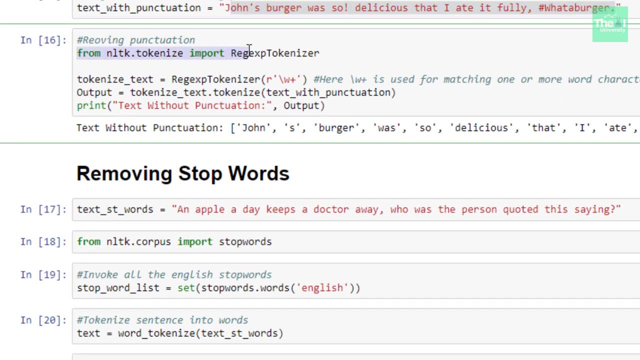 removing the punctuation after the word tokenization is done. okay, and the way I'm doing it here is I'm again importing a library which is regex-p-tokenizer- okay from nltktokenize okay. next, I created the object of, you know, regex-p-tokenizer- okay, and 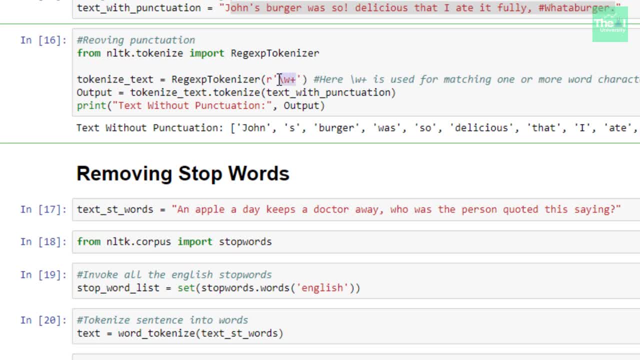 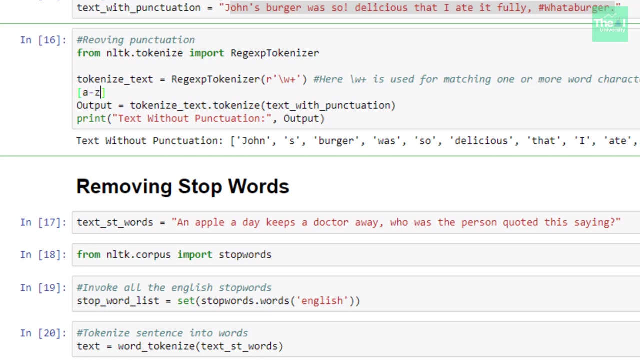 past this particular term which is slash w plus as an argument. So here w plus, slash w plus matches one or more word characters And it is same. as you know if you've already learned about a regular expressions, it is same as this term. okay, 029,. so this particular. 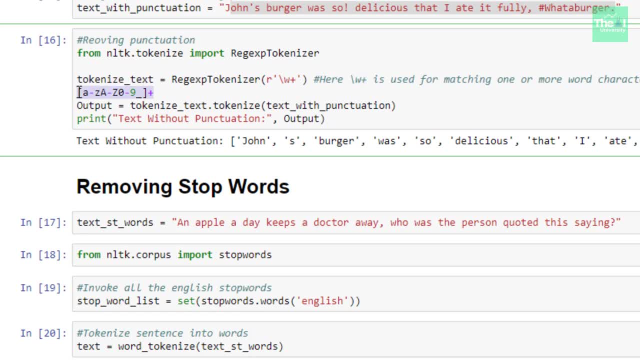 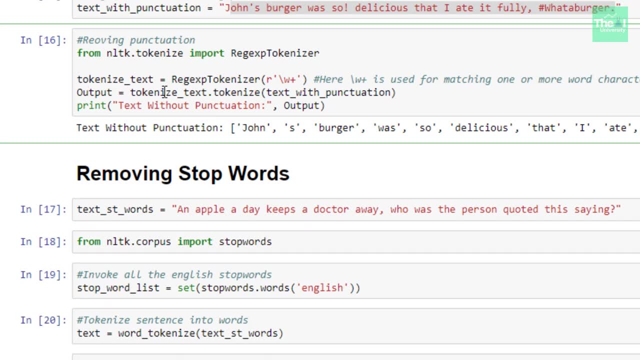 term represent this in regular expressions. Okay, so remember that Now, and what I? in the next line, what I did was I just used this tokenizer, okay, tokenize, underscore text, dot. tokenize and parse past this particular text as an argument to it. okay, and then printed the output here. so 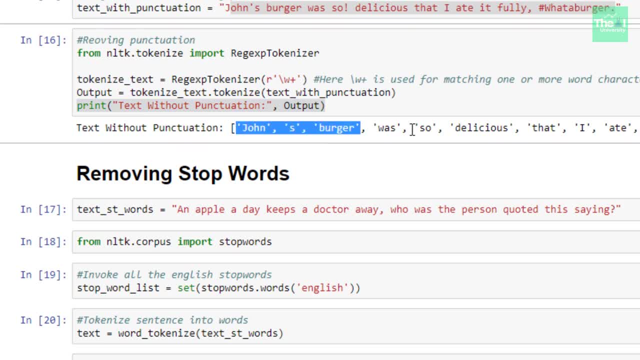 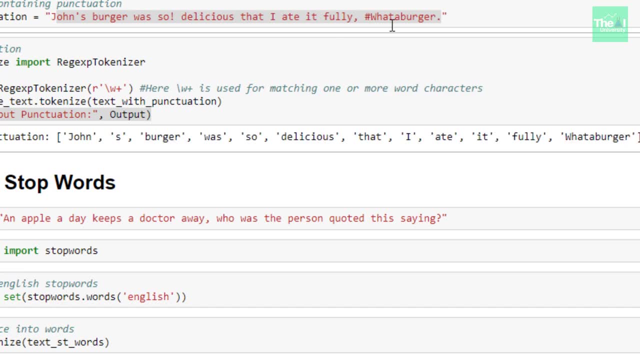 if you see the output in this list, you won't find any punctuation marks. okay, so this has already been filter. all the punctuation marks like hash comma, explanation mark, apostrophe, all these are filtered out from this particular sentence or text. as you can see here, all of the punctuations are removed, okay, so. 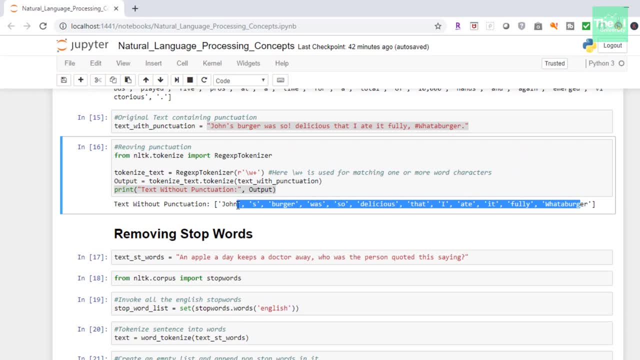 folks, this is it for this video. to conclude, I explained that tokenization in detail in this video and covered some of its variations, like word and sentence tokenization. so let me ask you a question from today's video: when does it is preferable to remove punctuation after doing tokenization or before doing? 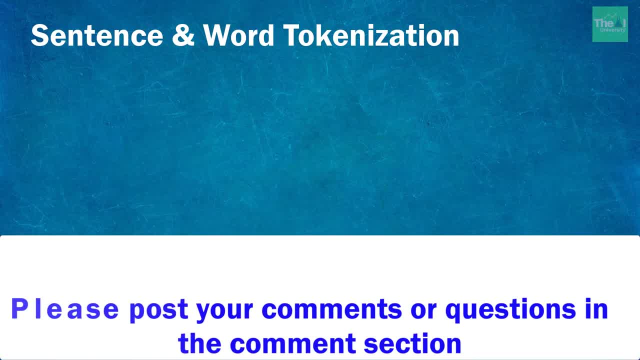 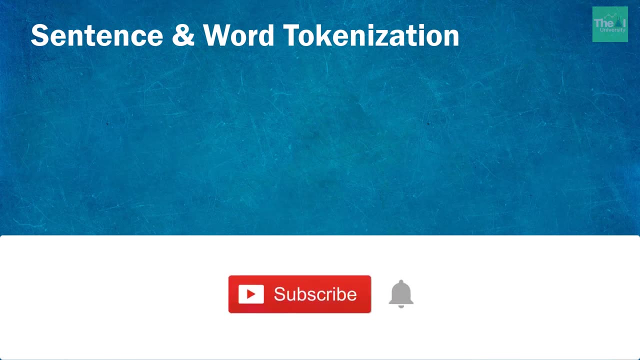 tokenization. please post your comments in the comment section given below so that I can get a chance to incorporate your feedback. you can also ask your technical questions in the comment section. I will be glad to answer your questions if you are watching this video and you are not already a subscriber to.